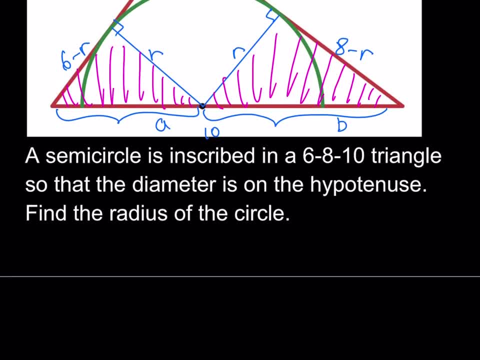 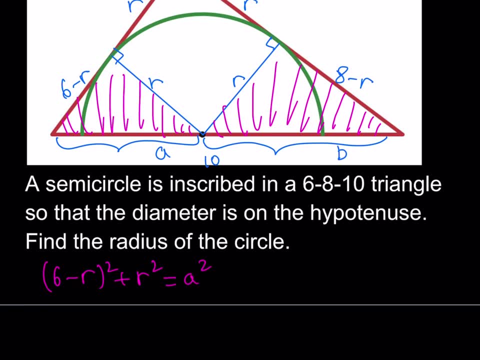 method. Let's go ahead and continue. So first I'd like to write 6 minus r squared plus r squared is equal to a squared, So this allows me to basically expand it right, And this is going to become 10.. So I'm going to write 6 minus r squared plus r squared is equal to a squared, So this allows me to basically expand it right, And this is going to become 10.. 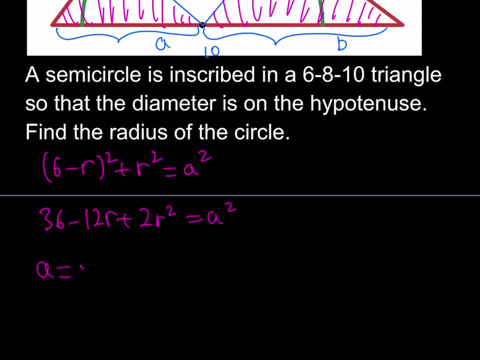 to r squared. So what I can do is I can basically square it both sides and get the a in terms of r. So that's going to be my first step. My second step is going to involve getting the b in terms of r, and then we'll put it, put it together. I'll show you how to do that. 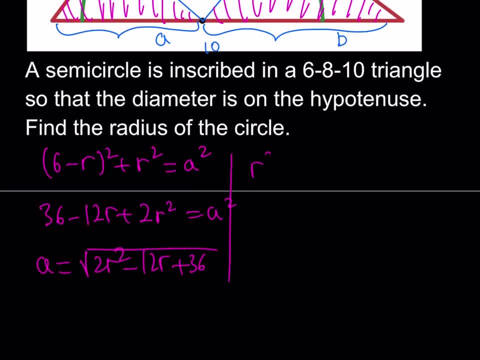 So the legs are r and 8 minus r, So it's going to be r squared plus 8 minus r squared is equal to b squared. From here we get r squared plus r squared, which is definitely 2r squared minus 16r. 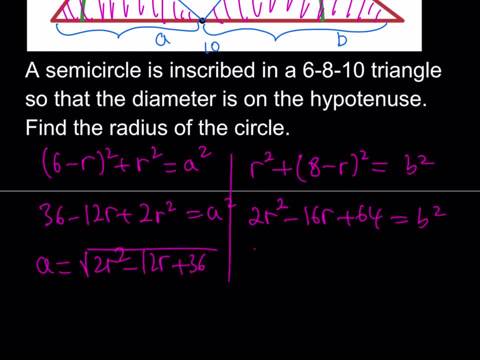 plus 64.. That should equal b squared. If you square it both sides, just like a, similarly, we're going to be getting the value of b, and that should be this one. So now I got a and b and I'd like to put it together. And how do I put it together? Well, they make up the hypotenuse right And the 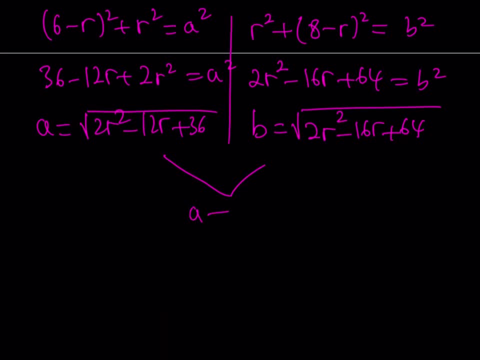 hypotenuse is 10.. So that means that a plus b is equal to 10.. So that's how we put it together. So let's go ahead and write that down as an equation, And obviously this is a radical equation. but guess what? We're going to turn this radical equation- which is very radical, by the way- 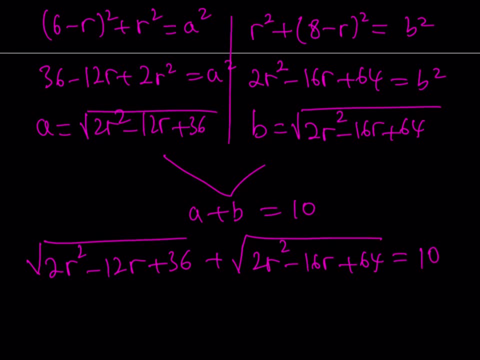 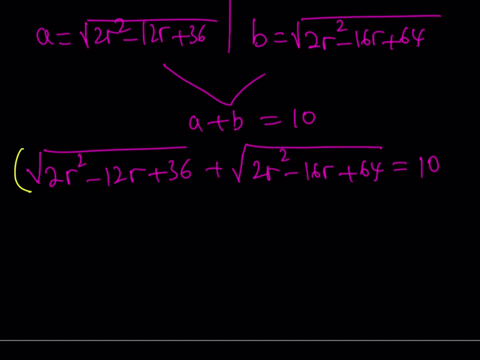 right, We're going to turn this into a quadratic equation. How do we do that? Well, we're going to square both sides. Let's go ahead and do it, But before we square both sides- I think this would be meaningful- Let's go ahead and simplify this a little bit, tiny bit. So what I'd like to? 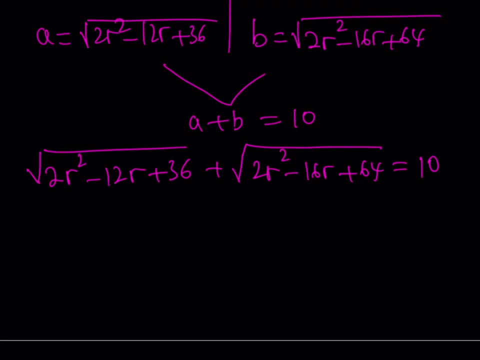 do is I'd like to take out the 2 which is going to come out as a square root of 2.. So I'm going to have the same term, but this time the 2s are dropped right, And then I have r squared minus. 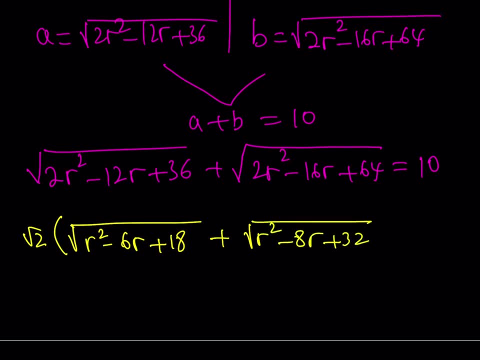 8r plus 32.. Everything is divided by 2. basically right, I divide everything by 2.. And this is 10.. So what I'd like to do is divide both sides by root 2.. And you know that we can rationalize. 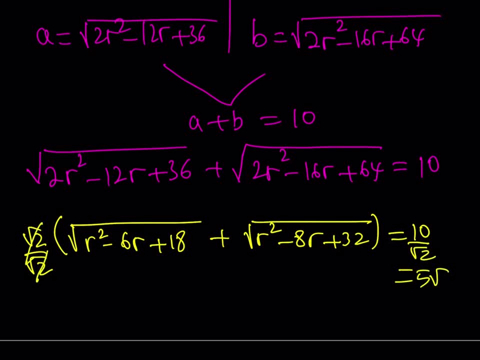 the denominator, And this is going to equal 5 root 2.. Beautiful, And of course, this expression is squared, And this expression is also squared. Let's just square both sides. Okay, you get the idea right, Hopefully, When I square both sides. 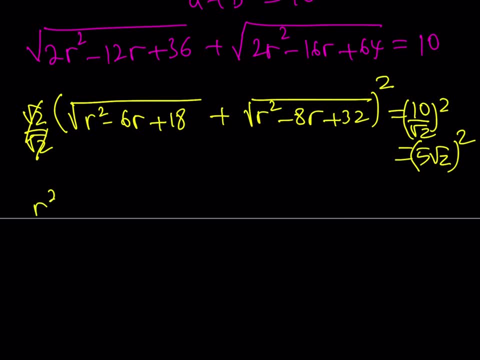 I'm basically getting the, the first expression, r, squared minus 6r plus 18.. And then I'm getting r squared minus 8r plus 32.. Okay, I'm going to call this a and I'm going to call this b, because 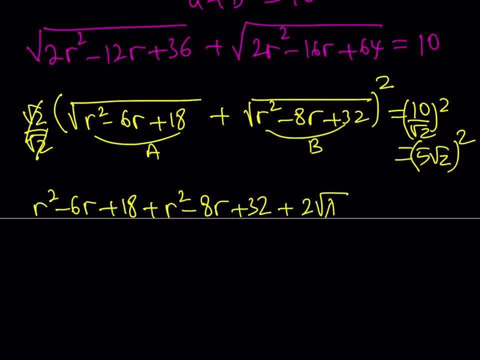 I'd like to do a little manipulation here and then take care of a and b later. Okay, so let's call those a and b, And that's the term that we get from the middle. And if you square 5 root 2, you'll be. 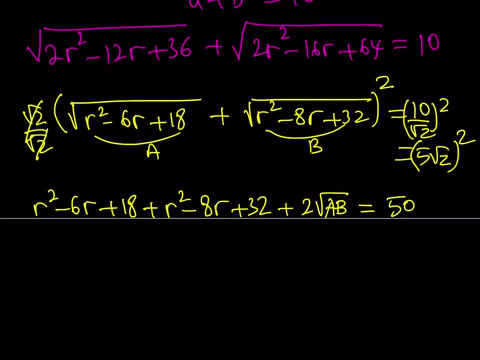 25 times 2, which is equal to 50.. Nice. Now, what makes it real nice is that 18 plus 32 is equal to 50. So those constant terms cancel out, And what do we get? We get 2r squared. Let's write that down. 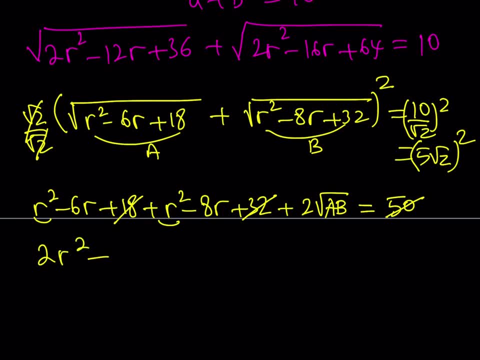 minus 18.. Not 18.. 6 plus 8 is equal to 14, right Yeah, arithmetic is kind of like my weakness, I guess Plus 2ab, square root of 2ab, is equal to zero. Obviously, I'd like to isolate these times. This is 1 by x, So you can use the square root of x. square root of x equals 1.. So all you have to do is take your numerator and write down your denominator. and write down your denominator. and write down your denominator. 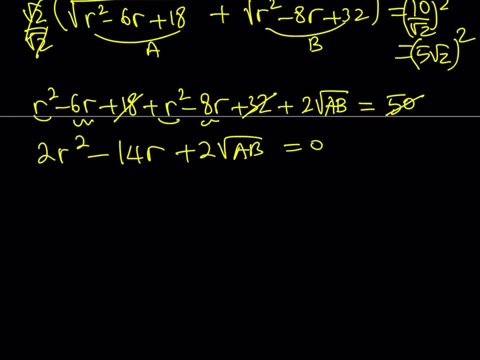 and write down each of those as you see. So anyway, this is really easy. It's really easy, That's. all is equal to 0.. Obviously, I'd like to isolate 2ab here, so let's go ahead and isolate it, but at the 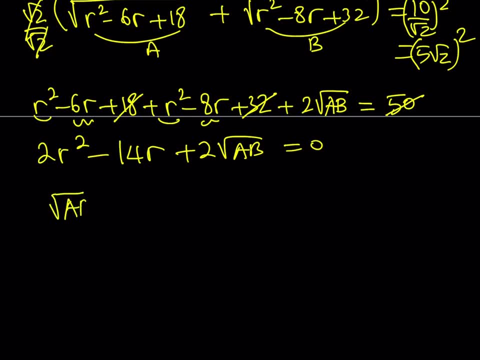 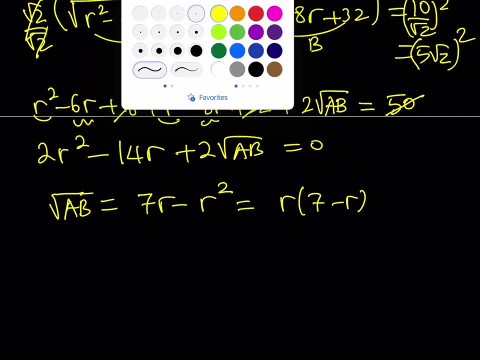 same time, divide everything by 2.. So this gives us something like: the square root of ab is equal to 7r minus r squared. Now I'm going to square both sides, but it would make sense if you wrote this as r times 7 minus r, because it's easier to square that way. So let's go ahead and square. 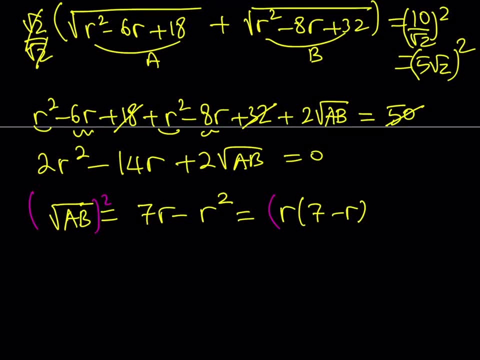 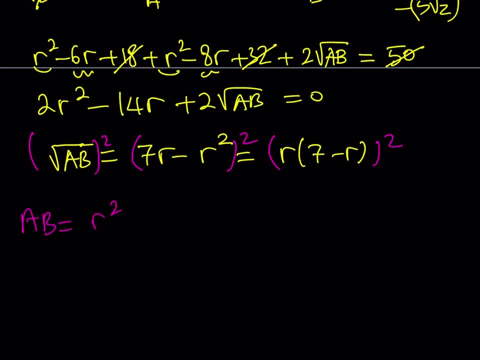 both sides here one more time. So then we get this and that and of course this is squared as well. So ab is going to equal r squared times 7 minus r squared is going to be 49 minus 14r plus r squared. 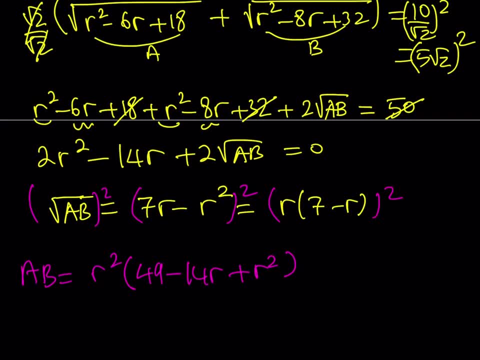 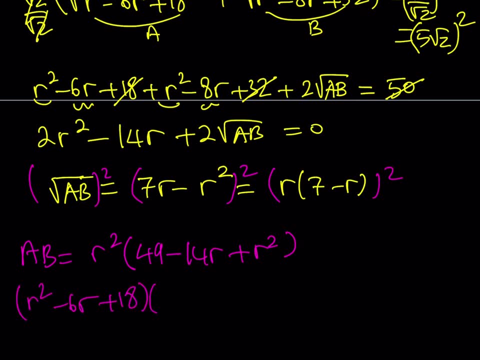 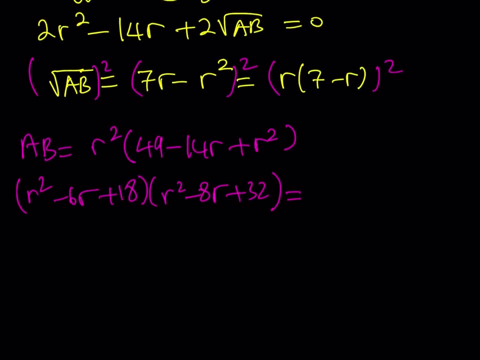 Okay, cool, Now I gotta go back and substitute a and b. a is equal to r squared minus 6r plus 18, without the radical of course, and b is equal to r squared minus 8r plus 32, and this product is supposed to equal that product. Let's go ahead and. 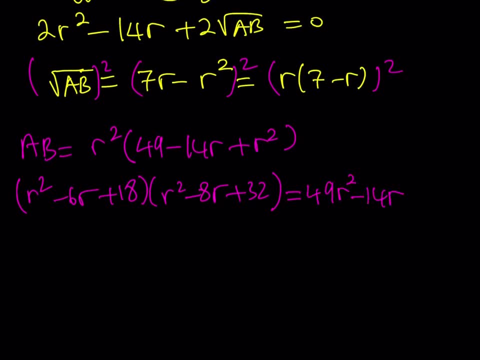 expand it: 49r squared minus 14r cubed, plus r to the fourth. Now this looks like a quartic, but it's actually a cubic, because if you multiply r squared by r squared, you get r to the fourth, and then you're going to distribute the whole thing right. You're going to be getting some r. 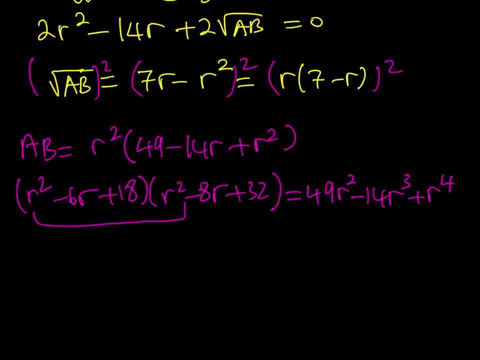 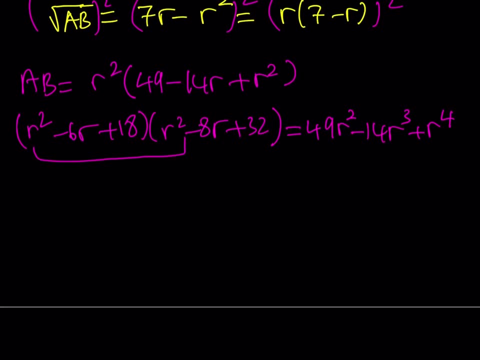 squared r, cubed, so on and so forth. I'm going to save you the trouble here, because it's kind of time consuming, and I'll basically give you the answer From this equation. a lot of things are, and you're going to end up finding the r value as 24 sevenths. Cool, That basically concludes our. 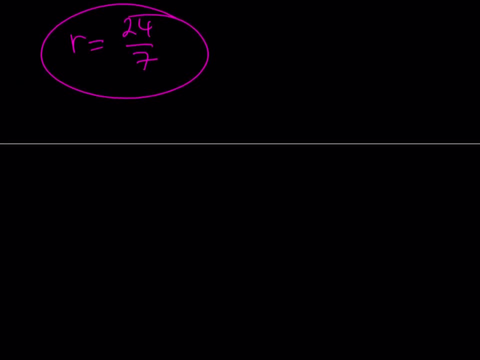 first method. So let's go ahead and look at the second solution method. Now, what does the second method involve, right? Well, the second method involves another tool that we use a lot in geometry, and that's called similarity. Now let's go back to our picture and see what that looks like. 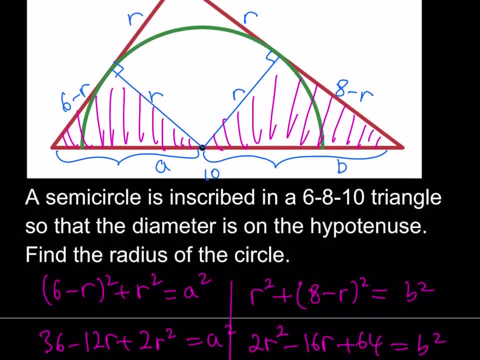 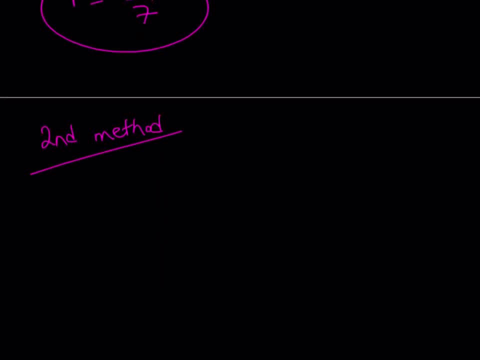 right. So here the original one, and we can actually kind of sketch a real quick one like this one. It won't be real nice, but I think it'll do, at least for our purposes. So basically we do have the 6, 8, 10. 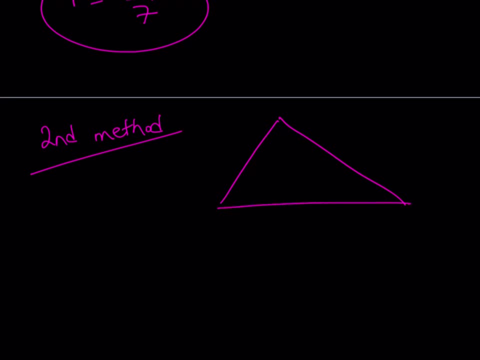 triangle right and inside it I basically have like a semi-circle that is basically inscribed like this right, Something like this. Is that good, Okay? so what I'd like to do is I'd like to find the r right. So here's how similarity works. So this is 6, this is 8 and this is 10.. 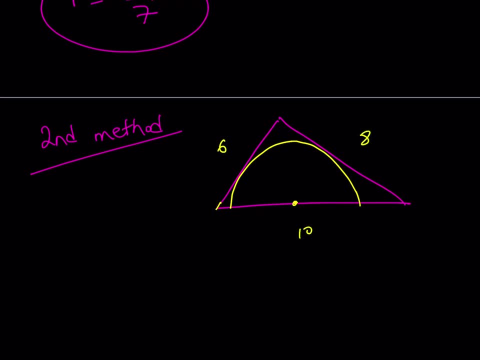 Okay, cool. Now, when I made those connections, I found that this was an r and this was also an r. You know that it could make it nicer, but that's okay, No worries. Now here's how I use similarity. Notice that this is a 90 degree angle and this is a 90 degree angle, And remember the triangles. 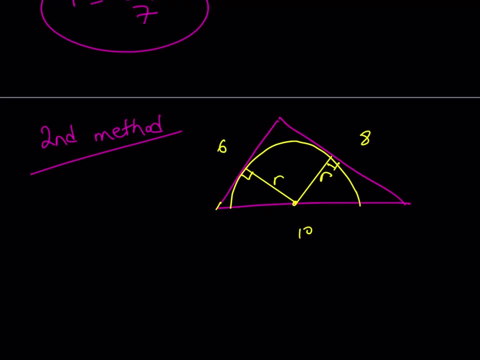 that we shaded before, Those triangles are similar. Why, If this is a 90 degree angle, which is- and let's call this alpha and let's call this beta, So we know that alpha and beta are what Elementary right? They add up to 90.. Okay, cool. So what's so cool about that? Well, here in this. 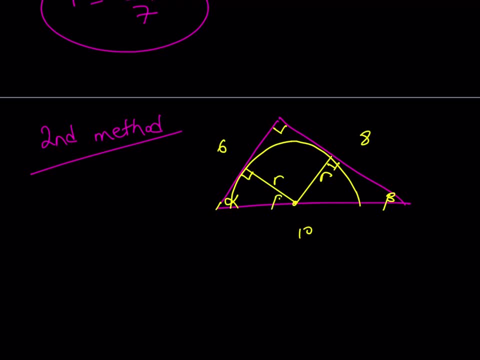 little triangle, alpha and beta also add up to 90. So therefore, this is beta and this is alpha. In other words, these two triangles. I can just dot them, not shade them completely, But these two dotted triangles are basically similar. So how do you use similarity, Similarity? 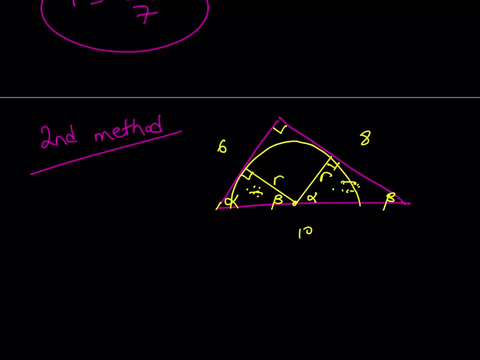 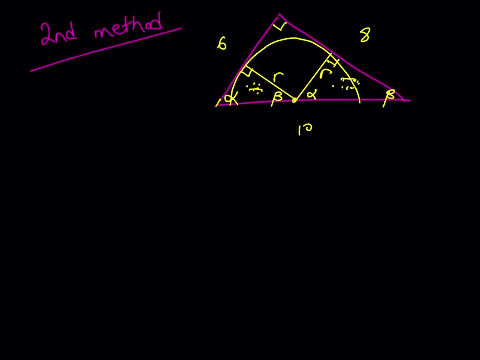 works off of ratios. And remember, this is the second method and you are supposed to compare these two methods. Which method is easier for you or which method do you like better? It doesn't have to be an easier method, right? Okay, cool, Now here's how it works. We know that this is r This: 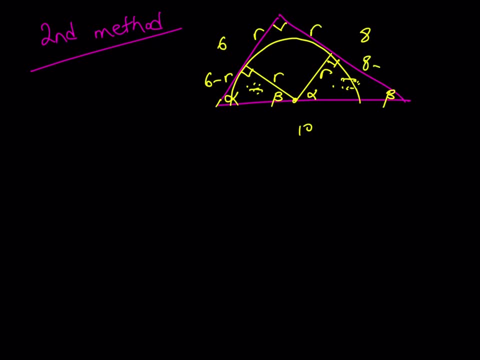 is 6 minus r, This is r and this is 8 minus r. Beautiful, I have everything I need. Do I need the hypotenuse? No, I don't, So I'm just going to use the legs. So how does this work? Start with. 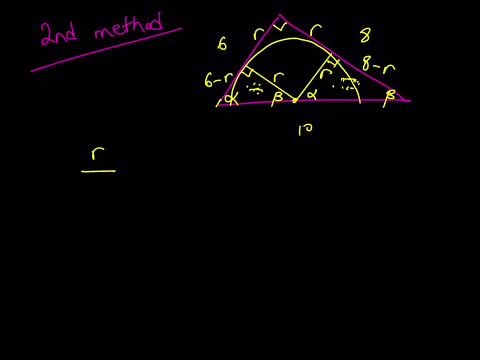 one of the triangles. What is across from alpha r. What's across from alpha in the other triangle? 8 minus r. Great, Okay, in the in the first triangle. what is across from beta? 6 minus r. What is across from beta in the other triangle, r. 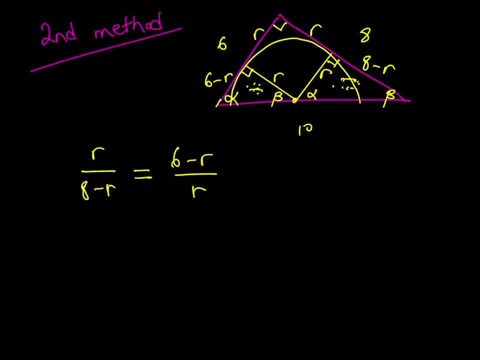 Beautiful, Awesome, Nice, Great. So I have a basic equation, Like: really I just need to solve this. Okay, let's cross multiply. r squared is equal to: If you multiply 8 minus r and 6 minus r, don't you get something like r squared minus 14r plus 48?? Because you know some. 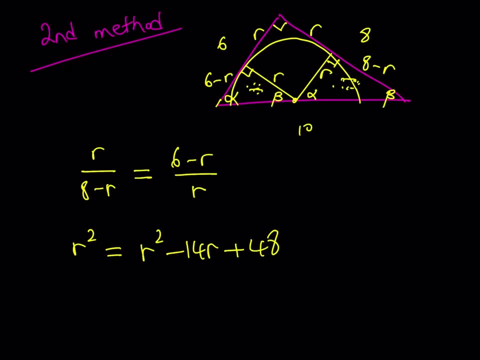 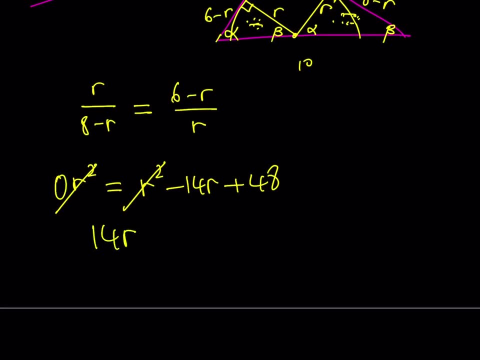 terms, cancel out Whatever. Oh r squared cancels out Beautiful, As if I didn't know that, right, r squared cancels out and you end up with zero Nice. So now we get 14r. if you end, If you add 14R to both sides, you get 14R equals 48.. 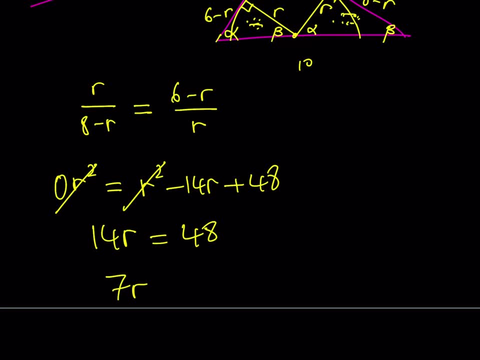 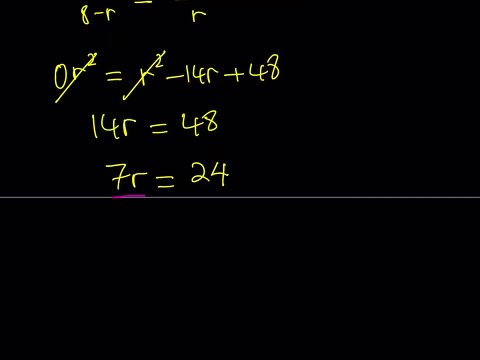 And obviously both sides. you can divide by 2. And this should give you 7R equals 24.. And in an effort to find R, basically if you go ahead and divide both sides by 7, you should be getting R equals 24 over 7..